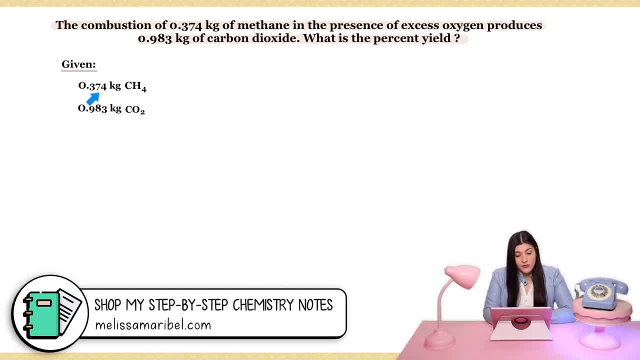 values. So I know that we have this amount for methane. By the way, what methane actually is, it's CH4.. And then it says for the presence of excess oxygen, but that doesn't tell me how much of oxygen we have. It produces this amount of carbon dioxide, So I know that well. 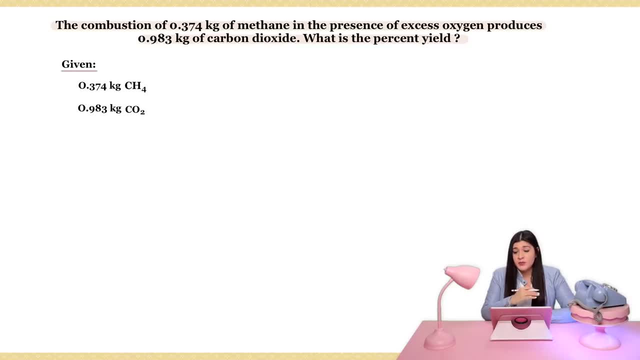 because it produces carbon dioxide. carbon dioxide must be our product, since it's being produced. So okay, I know that much. Now, what does that really tell me, though? Well, well, one, I know. I'm also looking for the percent yield. Now, for the percent yield we're going to need. 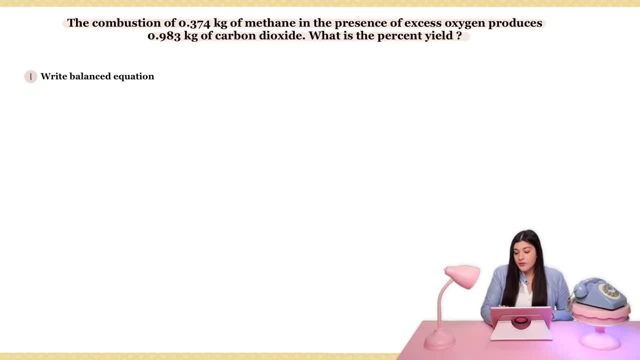 something known as the actual yield and the theoretical yield. So these are all the steps that we're going to talk about and go through. We're going to start off with writing the balanced equation, Then we're going to find the theoretical yield by doing a bit of stoichiometry And then 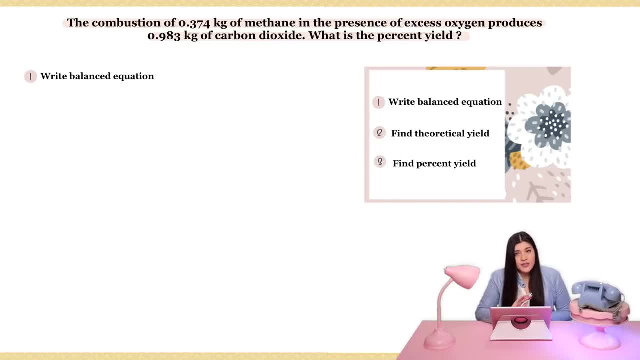 lastly, we'll find the percent yield by doing a bit of stoichiometry, And then, lastly, we'll find the percent yield. So I'm going to start off with just writing the balanced equation. Now, there's several hints in this question. One: you do have to know what methane is. It's CH4.. So, since I know 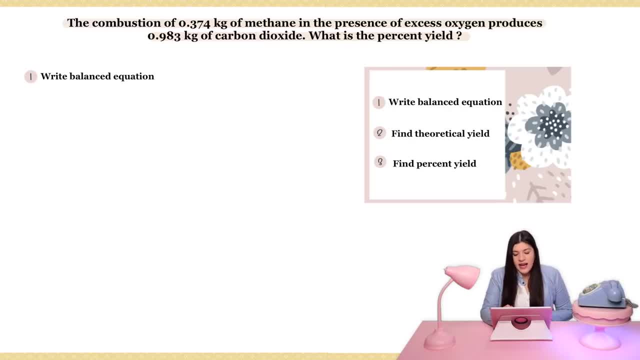 okay, that's methane, CH4.. And plus, this is telling me there's an excess of oxygen and it produces carbon dioxide. All of these are hints. The other huge hint is just the fact that it says it's combustion. If it's combustion, well, I now know the type of reaction it is And I know all the 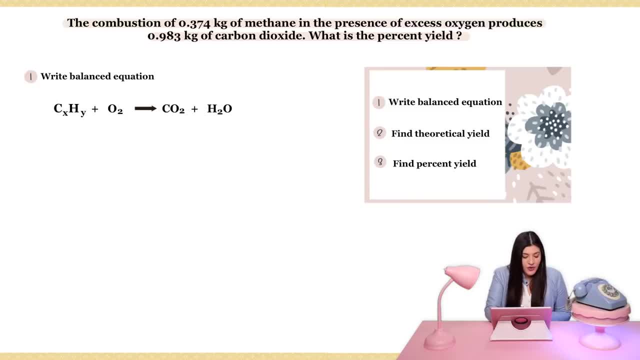 parts of this equation. So, in a combustion reaction, recall that we're going to have something known as a hydrocarbon. What a hydrocarbon is? it's just a molecule that consists of only hydrogens and carbons. So that's our methane in this case, And what never changes. 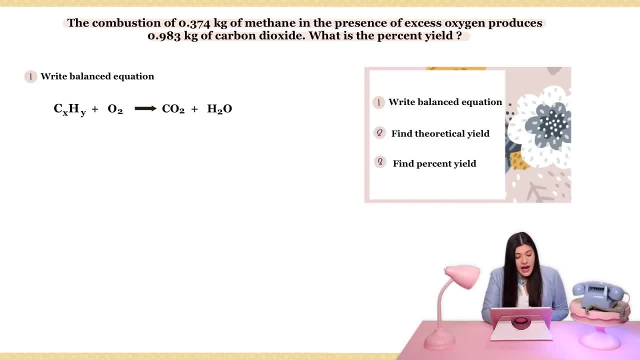 is your reactant and your products. So you're always going to react this with O2.. That's the excess O, or oxygen, right O2.. And then oxygen will not exist just by itself. It's a type of diatomic molecule, meaning it exists in pairs. So that's why we have that O2.. Next it's going to 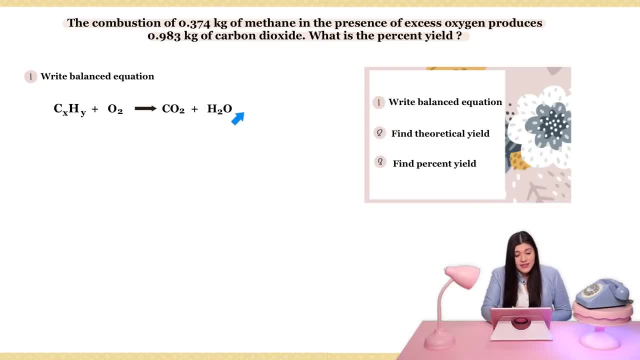 produce carbon dioxide and also water, just because this is a typical combustion reaction. So, as I mentioned, this never changes. This part never changes. The only thing that changes is the hydrocarbon that you're initially given with. So in this case, I know that I'm going to start off. 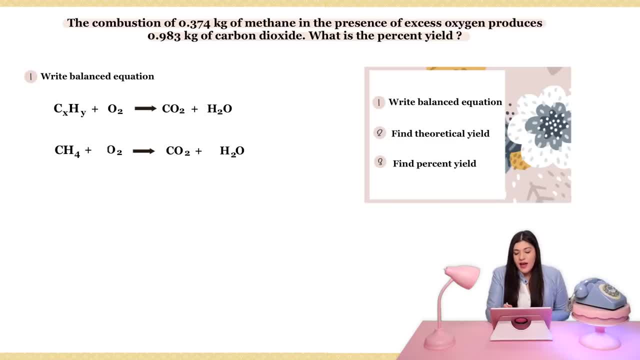 with our methane. that's provided. I'm reacting that with the excess oxygen- so O2, and we'll produce carbon dioxide and water. So now that we have that, we're going to react this with O2.. We have that, Let's just balance this out. So what I like to do with balancing is just write out. 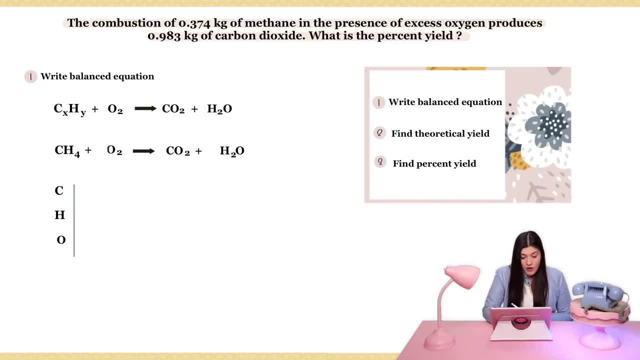 every single element individually on either side for our reactants and our products, And I'm going to identify how many of each element we have on either side: on the left side, which is the reactants, and the product side, which is the right side, which is the product side. So in this, 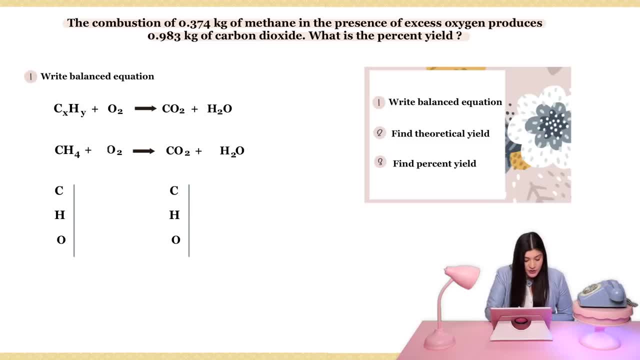 case, I have one carbon on the left side or the reactant side, And then for hydrogens, I have four right. Because of this subscript, I know that I have four. Next, for oxygen, the subscript tells me there are two oxygens on the left. I'll do the same thing. 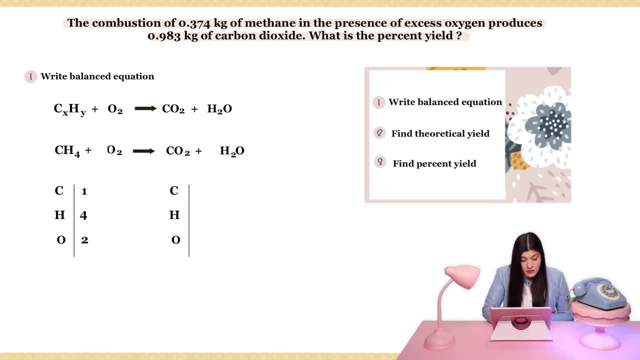 for the product side. So, looking here, there's only one carbon, So one carbon. Next, for hydrogen, there's two due to this subscript, So two hydrogens, And be aware of your oxygen. here Some people may say, okay, there's only two oxygen. That would be wrong, because don't forget about 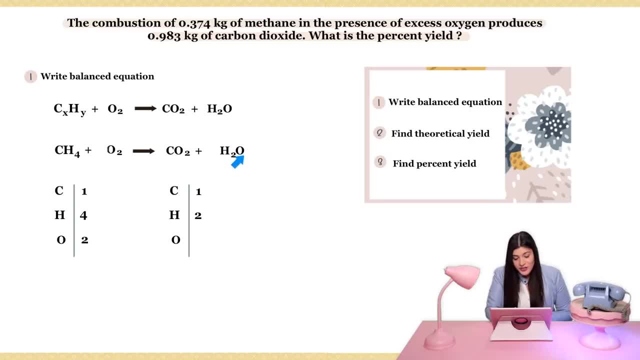 this other oxygen, So we have two plus this additional oxygen, So there's actually three, So three oxygens Okay. So just a rule of thumb for balancing: always leave oxygen to the very end, because it tends to kind of work itself out or get a little bit confusing if you start there. So I'd say start. 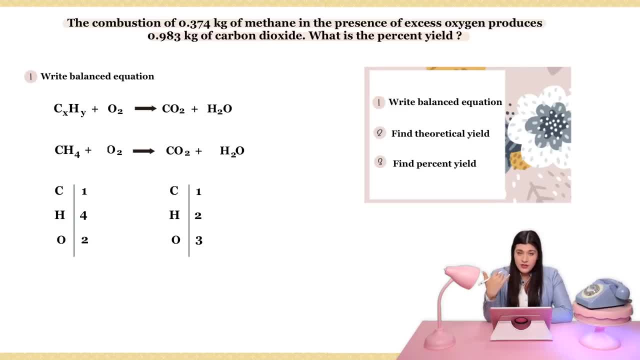 off with anything other than oxygen, So I would typically start off with carbon. However, carbon in this case is balanced already, So now I'm going to move on to hydrogen. So, okay, I need two more here, right, Because this is four and this is two, So I'm actually going to place a two in front, so 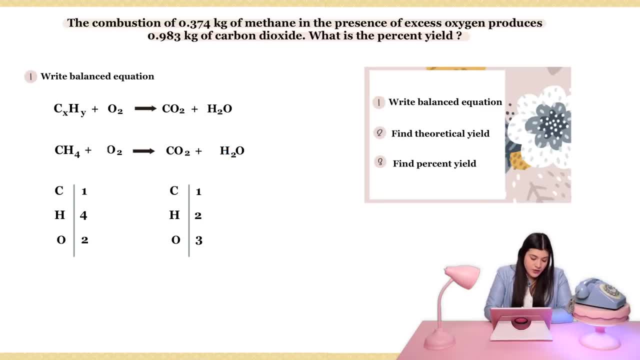 it can then multiply with that hydrogen. So I'm going to put a two in front so it can then multiply with that hydrogen. So I'm going to put a two in front so it can then multiply with that hydrogen And become four. So that's exactly what I'm going to do. I'll place a two in front Now when I do. 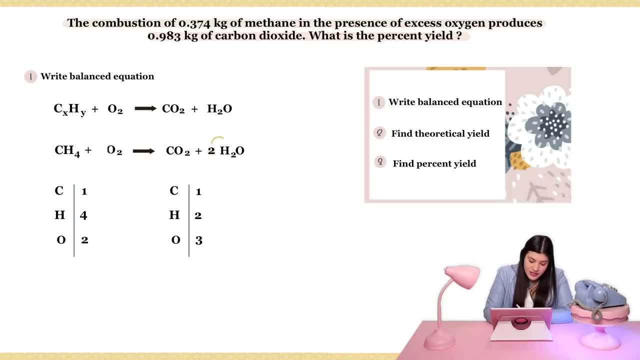 that it's like I'm distributing now This two into the hydrogen and to the oxygen. So I know well, the amount of carbons didn't change because I didn't place anything in front of this carbon. So I know carbon is still one, But the amount of hydrogens does change because I multiplied two. 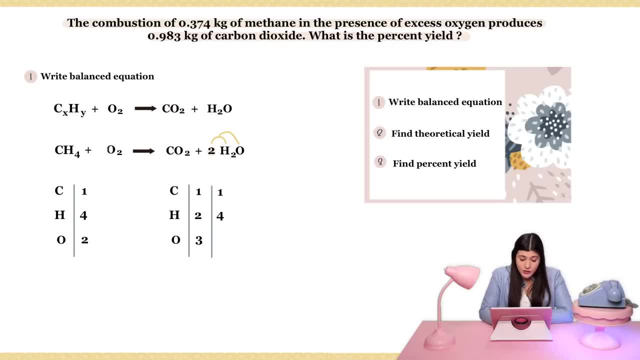 times two, which now gives me four. Our oxygen will also change because we have two times- well one, since there's no second. So that's exactly what I'm going to do. So I'm going to put a two in front Now. when I do that, it's like I'm distributing now This two into the hydrogen. So I'm going to put a two in front Now. when I do that, it's like I'm distributing now. This two is two. So I'm going to put a two in front Now. when I do that, it's like I'm distributing now This. 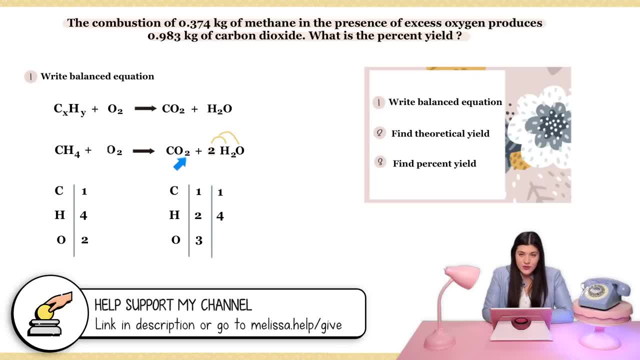 is still one, Since there's no subscript there really. so two, But that's not it, because I still have an additional two here. So two plus two gives us four. So now we have four oxygens. So now that we have this, the last thing we have to do is just balance out our oxygens. So let's keep going So. 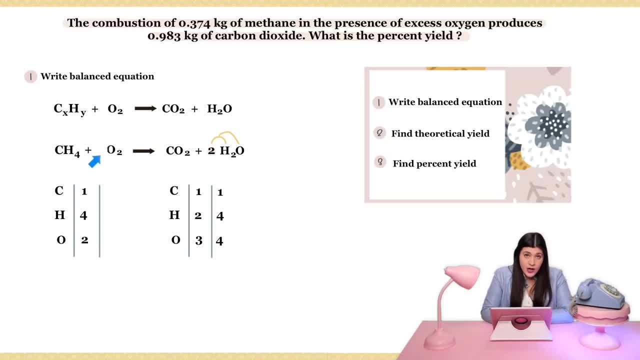 then now I'm going to look back here and say: well, what number do I have to place here to multiply with this two subscript, to give me four. well, two times two. so I'll place a two here. these two would then multiply and that's gonna give me four oxygens. 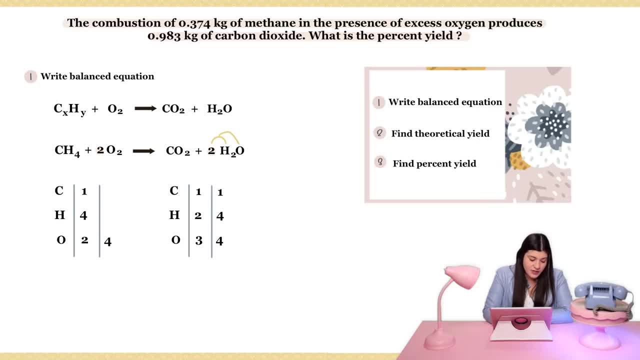 while nothing changes for carbon, since I didn't place anything in front of CH4, and then nothing changes for hydrogen, since, once again, I didn't place anything in front of CH4. so now that we have our balanced equation, let's go to step two, which is finding the theoretical yield alright. so with this type of question, I 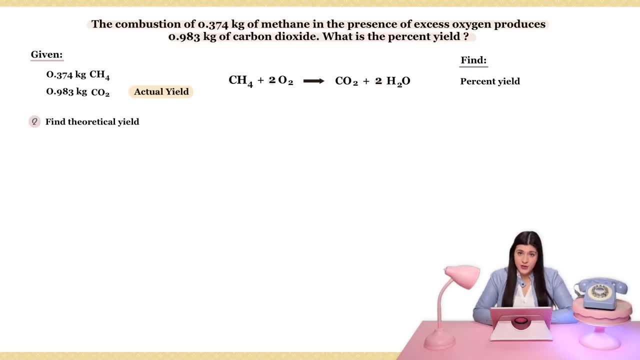 know to find a theoretical yield, because well one, it's telling me to find the percent yield, and the formula for the percent yield is actual yield divided by the theoretical yield. so I need it now. the theoretical yield is found by well identifying the limiting reactant and in this question they actually tell you. 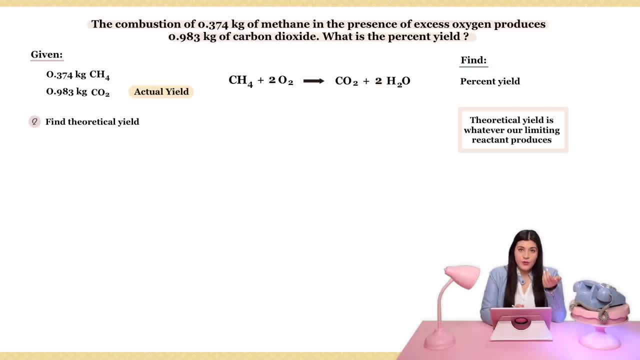 what the limiting reactant is already, because they tell you what's going to be produced. so they only give you one amount or one, yeah, one amount of our reactant. they don't tell you the amount for O2 plus. they tell you that O2 is. 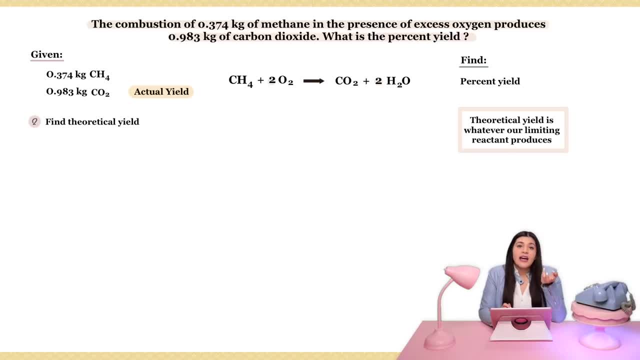 actually the reaction that you're producing and they're actually going to your excess reactant by just stating excess. Now, if you need to figure out or need to go over how to find the limiting reactant, I do have a video on that. You can find that right here, So definitely. 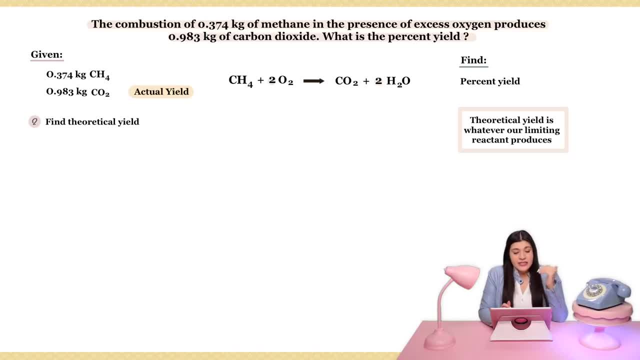 refresh your memory, because that is really important with this question. So, continuing on with just finding the theoretical yield, what I'm going to do is I'm only going to do this one, since I'm looking for the theoretical yield, specifically of the limiting reactant, which 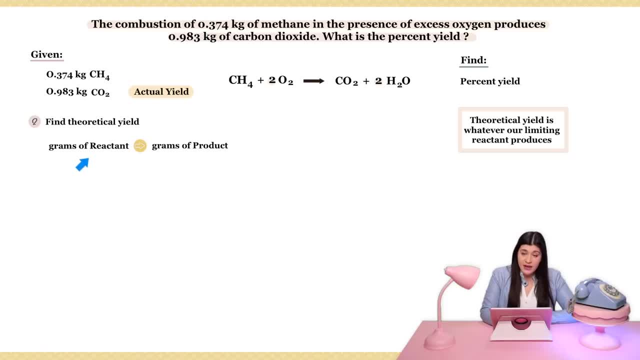 is methane. Well, I'm going to go from grams of my reactant to then grams of my product, which is carbon dioxide. right, Because this is our actual yield. I need the theoretical yield of the same product, which is carbon dioxide, But we have an additional step, just because I'm not starting with. 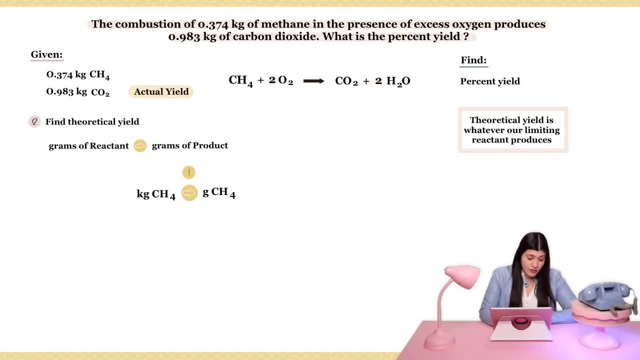 grams. I'm starting with kilograms, So that's actually what I have to start off with. I have to start with converting kilograms of methane to grams of methane by using the metric system, And then, from grams of methane, I have to convert kilograms of methane to grams of methane by using the metric system. 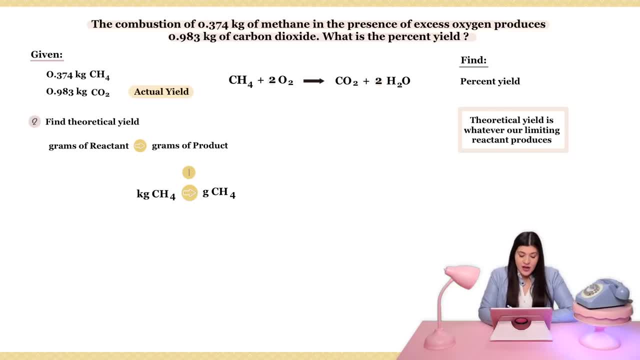 So I have to find my way to grams of our product or grams of CO2.. If you don't know how to do that, once again this is stoichiometry. Well, how you're going to do that is, you're just going to. 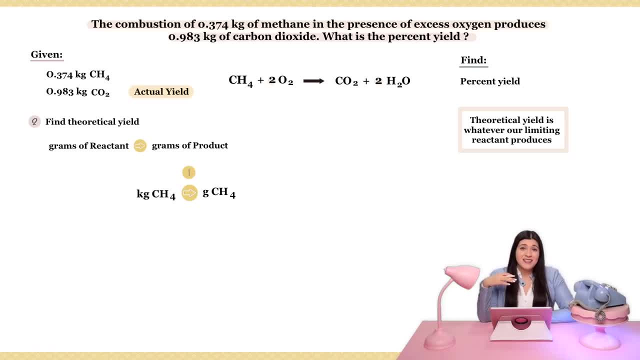 convert to moles Whenever you're not sure what to convert to. typically, like 99% of the time, moles is going to be your best bet, since all of the conversion factors equal moles. okay, Not in this case for kilograms, but at least when we're starting with grams. So what I'm going to do is 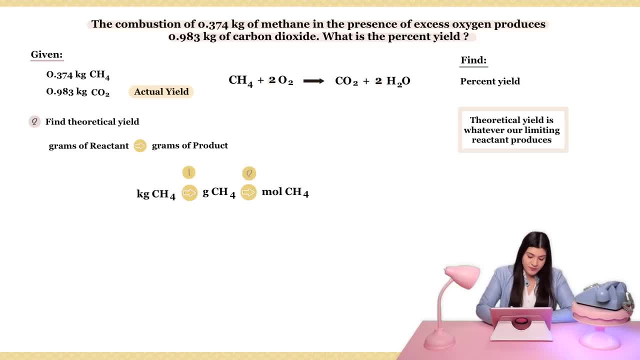 I'm going to convert to moles in this case. So I'm going to convert to moles And then now, since I'm at moles of methane, I want to do a mole to mole ratio to then get the moles of CO2,. 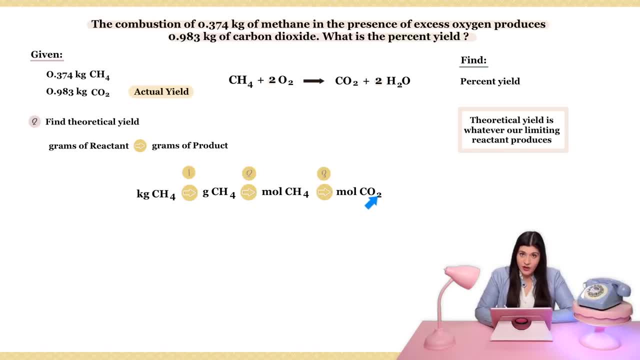 which is our product. So this just allows us to change the compound that we're looking at. And then, finally, I want to get back to grams, and I'll use the molar mass in this case to get back down to CO2, so grams of CO2.. So this is our plant. Now I'm going to keep going. 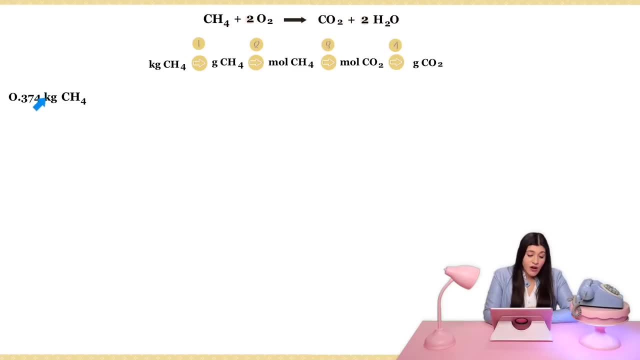 and let's just put everything together and do the math. So, starting off with the kilograms that we were given initially, this is the amount of kilograms I have for methane. now, what I'm going to do is I'm going to just convert this to grams. So this is our first step. 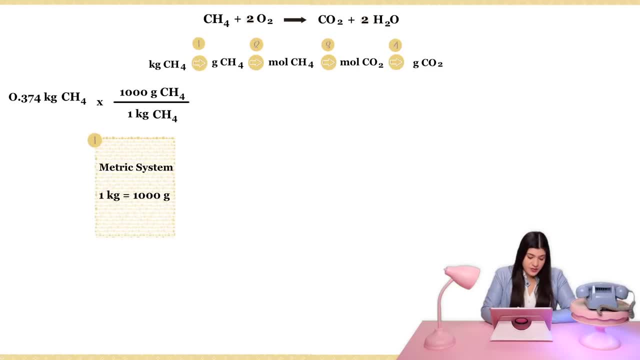 What I'm going to use is the metric system. So the metric system tells us that one kilogram is equal to a thousand grams. So, okay, I know that Now all I have to do is multiply. So these two would then cancel. So let's show that These two cancel. And then now I'm at grams of methane. Now. 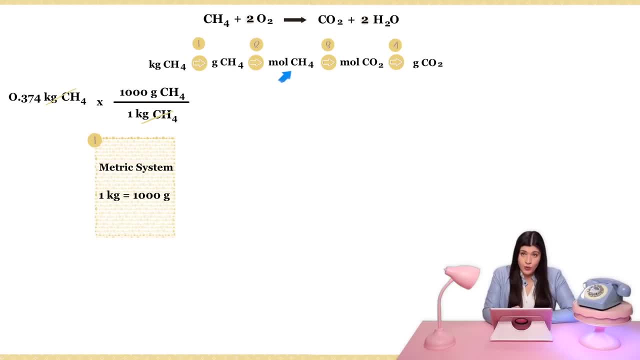 that I'm at grams of methane. I can then move forward to go to moles of methane. How I go from grams to moles is by using the molar mass of methane. So I know I'm going to use this molar mass. Remember how to find molar mass. All we're doing is looking at the individual masses. 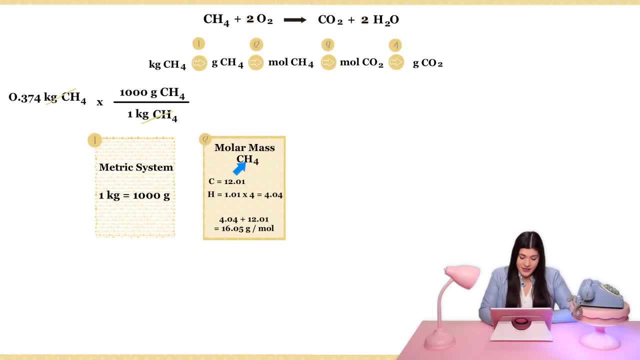 of every single element in this compound and then adding them together. So carbon is 12.01, and then hydrogen is 1.01, but there's four of them. So I'll multiply that by four and I get this. Then I'll add these two values together to get this as our molar mass. So what I'm going to 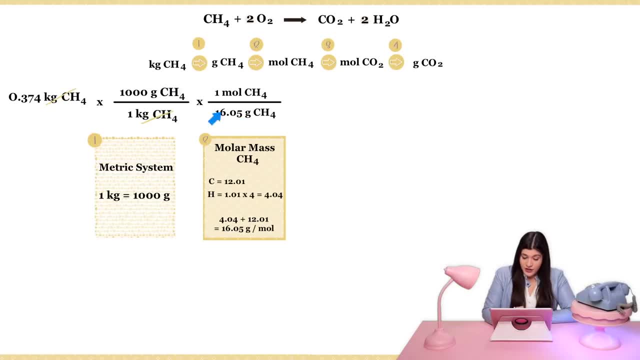 do is I'm going to use the coefficient so they can cancel. So these two units are aligned across from each other. So I know that those grams and grams of methane would then cancel, And that brings me to moles of methane. So I'm here. So, now that I'm here, I'm now going to move on to 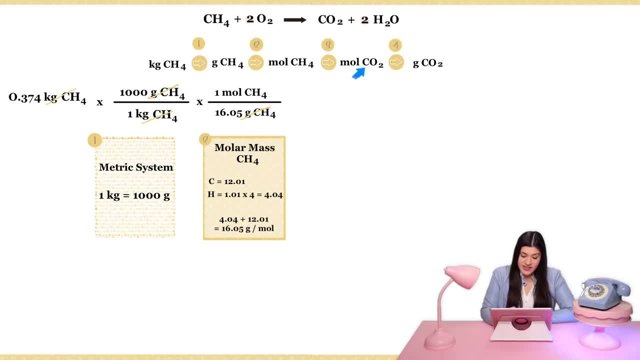 do a mole to mole ratio to get the moles of carbon dioxide. So, like I said, a mole to mole ratio is going to take place here. That's what allows you to go from moles of one compound to moles of a completely different compound. What I have to do is use the coefficient. So I'm looking at. 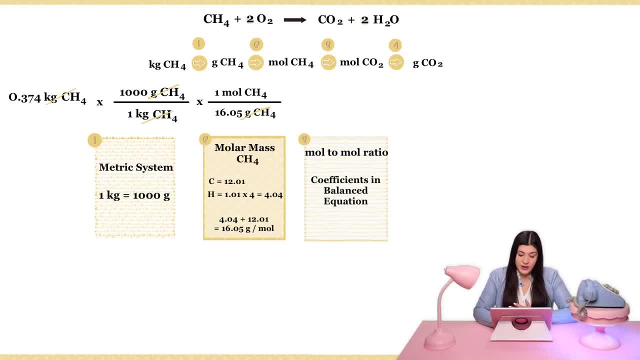 the balance equation and I'm looking at the coefficients involved in our balance equation. So it'll make sense once we do this. So what I'm looking at is looking at this balance equation. there's really a one here, So there's technically a one right here, and there's a one right here if. 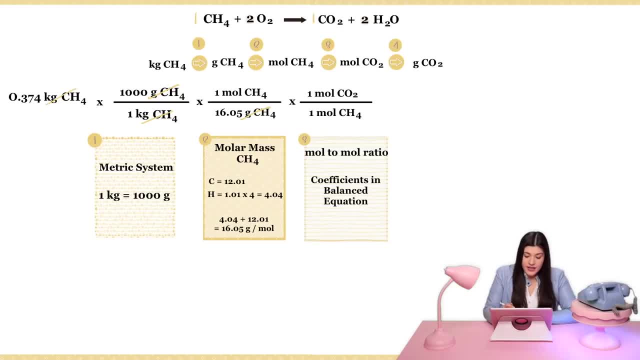 there's no other number that's being shown. So then I know well, there's one mole of methane and I'll align the units again so they can cancel. So those cancel. And then for every one mole of CO2, now that I'm at moles of CO2, I can then convert this to grams of CO2 by using the molar. 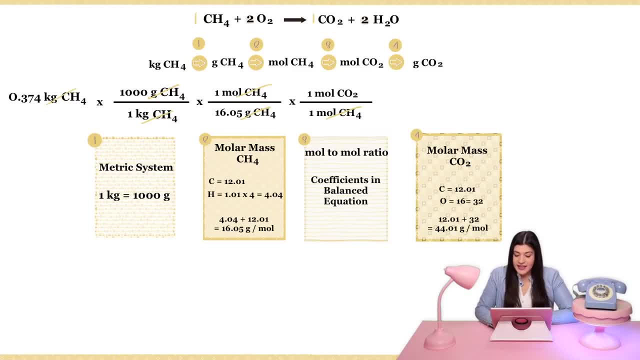 mass of CO2.. So once again finding the molar mass. I'm just adding this together. So then this is carbon 12.01, oxygen, And then I did multiply 16 times two. just a little note So. 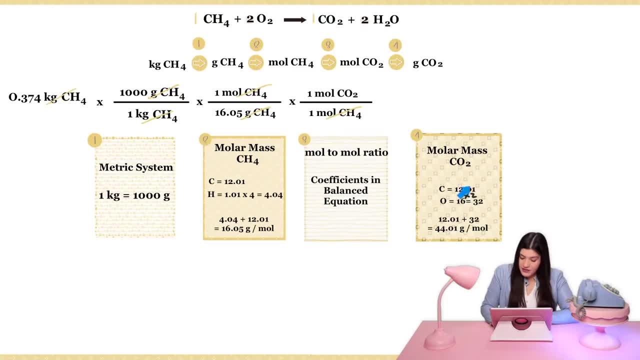 that's how I got that 32.. So multiply that by two And then add these two values together And this is our molar mass for carbon dioxide, And I'll place that here. So we're multiplying by it. I 'm multiplying by it because we're aligning once again the units across from each other, so they 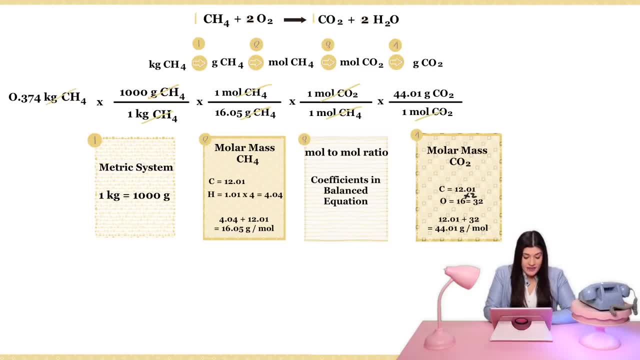 can cancel. So that's how you know where to place everything. And then, from here, almost done. I'm now going to multiply all of this together. So I'd multiply everything right across and then I divide by that: 16.05.. When I do that, I get this value, But I always have to worry about my sig figs. So 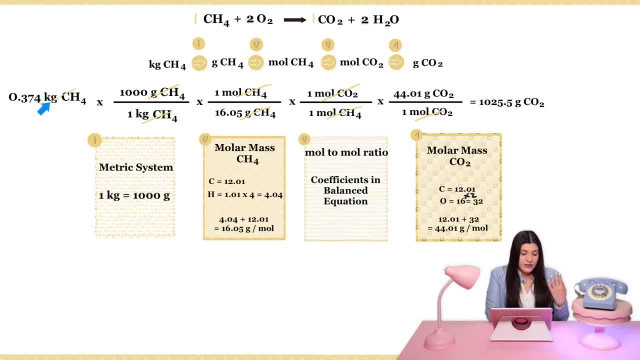 in this case, looking at what we initially were given, we were only given three significant figures. so I have to round a three sig figs. So I'm going to do that And then I'm going to add three sig figs. So I'm going to round up to this And remember, this is three sig figs because 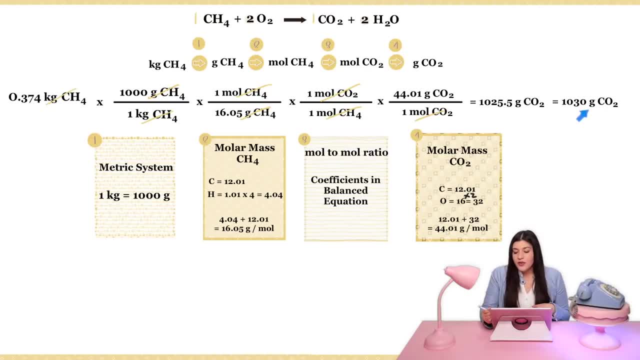 anything that doesn't have a decimal. it's a large number without a decimal. those ending zeros do not matter. So I only have three sig figs in this case: that one, this zero and three. So this is my theoretical yield. Okay, we found the theoretical yield. Now let's find our percent yield, Because 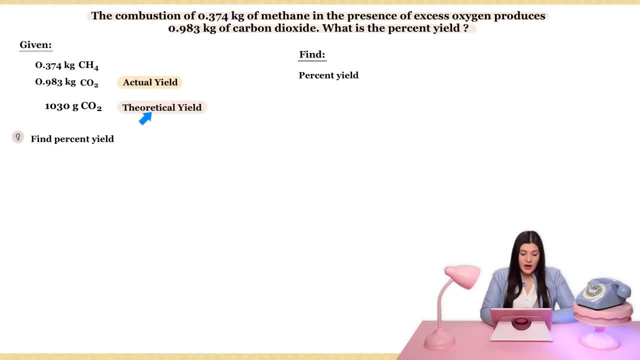 we have our actual yield and we have our theoretical yield. what we now have to do is plug this into the transfer function. we can plug it into our input. Okay, And that's the actual yield, Okay. So we can plug this into the transfer function, Okay. 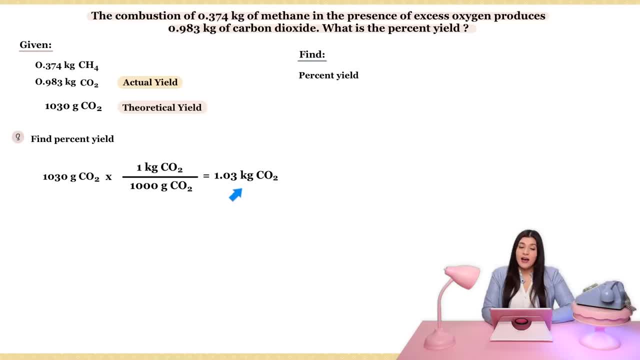 Okay to give me this amount of kilograms. so okay, i have my kilograms now. now that both of these are in the proper unit, the same unit, then i can continue. so our percent yield formula is our actual yield divided by the theoretical yield, and multiply that by 100, since it is a percentage. 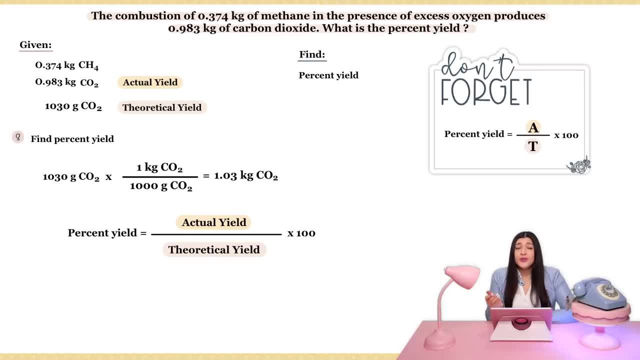 if you forget this- which please don't forget this- all you have to think of is percent yield. it's where it's at all right, so where it's at that's percent yield. so that's just a nice way to be able to remember this, just in case you forget this on your exam. so all we have to do now is 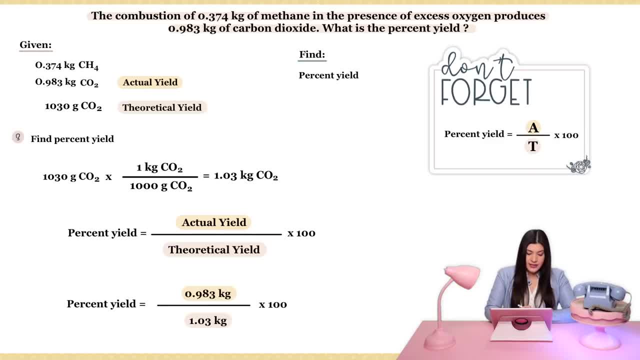 plug everything in. so i'm going to plug in the actual yield which was given and then i'll plug in the theoretical yield which we found using stoichiometry. divide these two values and multiply by a thousand and we get 95.4. that is our percent yield. let's move on to the next question. that asks: 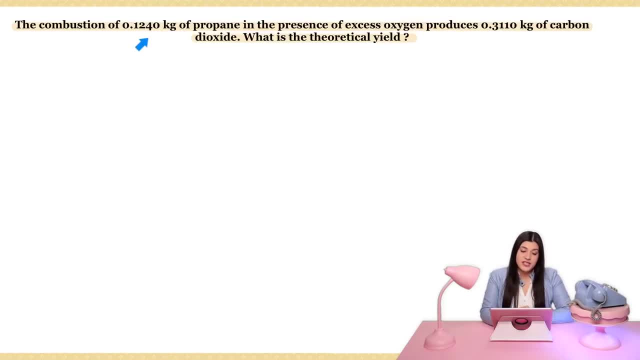 for theoretical yield, all right. so this question states the combustion of 0.1240 kilograms of propane in the price of propane expinding. we were going to be working at point four percent of this amount. so this number is the spiritual second year that it stipulates my真的很 value right now. 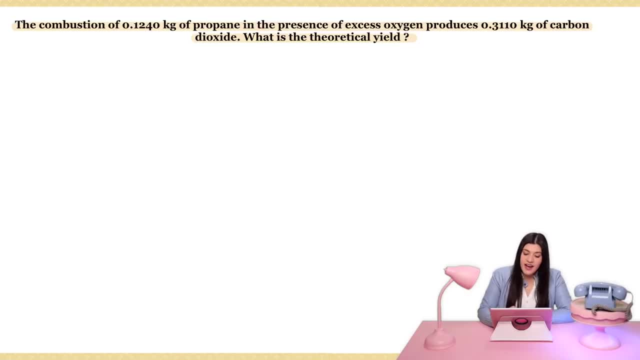 so now let me double click on what this number states. these numbers for us, in terms of: they account for: presence of excess oxygen produces this amount of carbon dioxide. what is the theoretical yield? So it's really similar to the previous one that we just did. 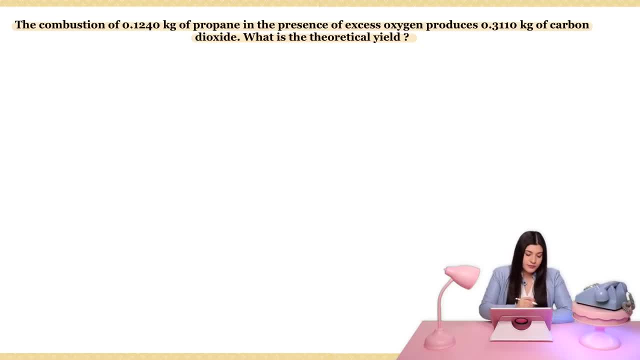 Let's once again identify what are we given and what are we finding. So we are given this amount of propane, and propane that's one to know, propane is C3H8, and then we are given again how much product we are producing. 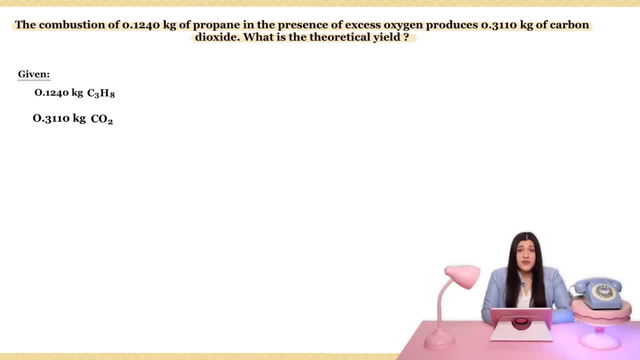 So we are given our actual yield. Is it relevant? Do we even need our actual yield? Nope. So this is extra information. there's no need to even use it in this case, because we're not asked to find the percent yield. So because we're not asked to find the percent yield, the actual yield isn't necessary in. 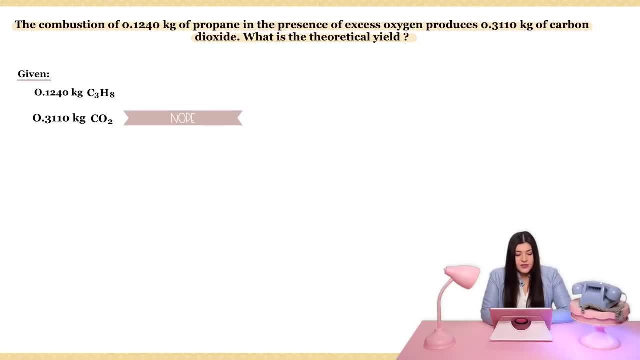 this question. So instead, all I'm using is just the amount of kilograms of our reactant or of propane, And then, of course, what I'm finding is our theoretical yield. The steps that we're going to take to find our theoretical yield are as follows. 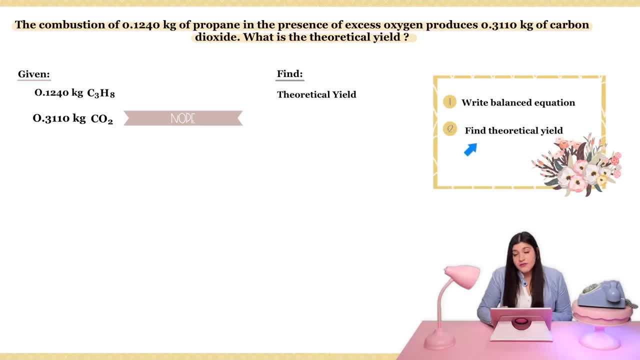 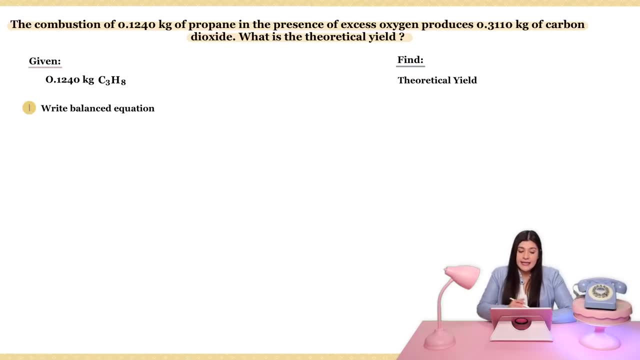 All we have to do is figure out the balanced equation and then find the theoretical yield with using stoichiometry, like we did previously. So let's start off with our balanced equation. Once again, this is a combustion reaction, So that means that the only thing that changes is this hydrocarbon, and everything else remains. 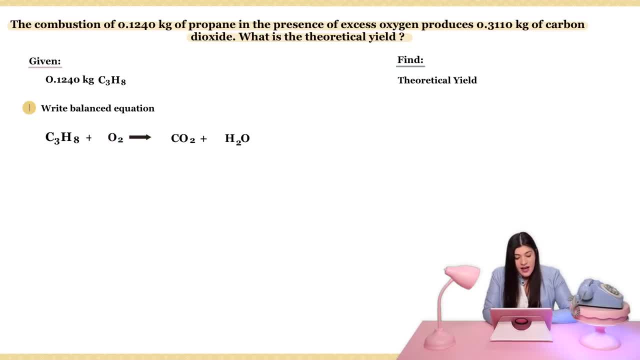 the same where we're adding O2, that's, our excess oxygen, And then it produces that carbon dioxide and water. So, doing this all over again, just balancing this out, Remember, we're going to re-evaluate, We're going to write all of the elements on either side and figure out how many of 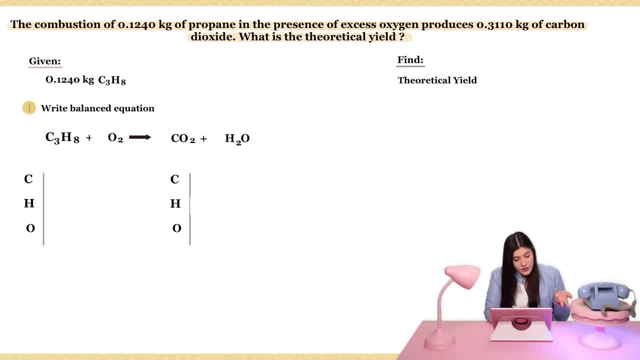 each element we have on either side and then balance them out. So, looking at carbon, on this side we only have three due to the subscript, So I have three carbons. Next, looking at hydrogen, there's eight, so eight hydrogens. 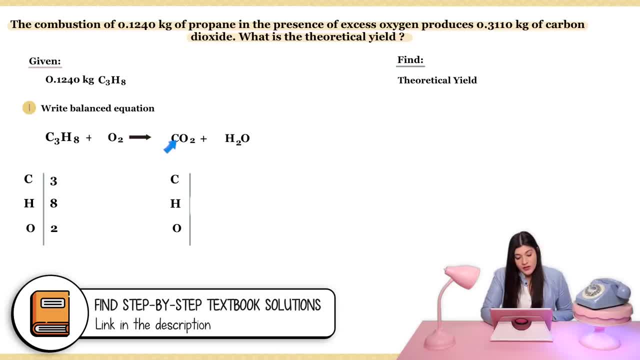 And oxygen. there's two. All right, looking at our product side, carbon. there's only one carbon here For, let's see, hydrogen. there's two because of that subscript, And then oxygen. Remember, there's actually three because we have two plus this one, so three oxygens. 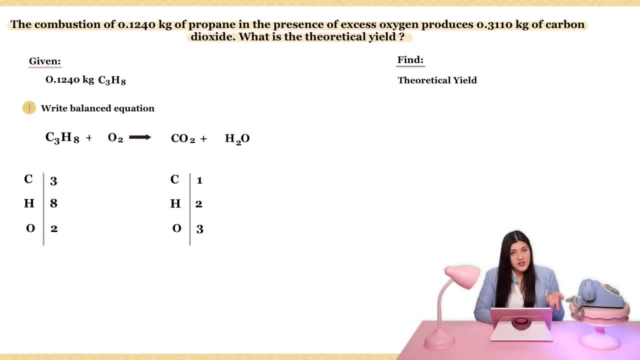 Always start off with, I'd say, anything that's other than hydrogen or oxygen. Always leave oxygen to the very end, because it makes it a lot easier. So I'm going to start off with carbon. So carbon: there's three carbons here and there's one carbon there. 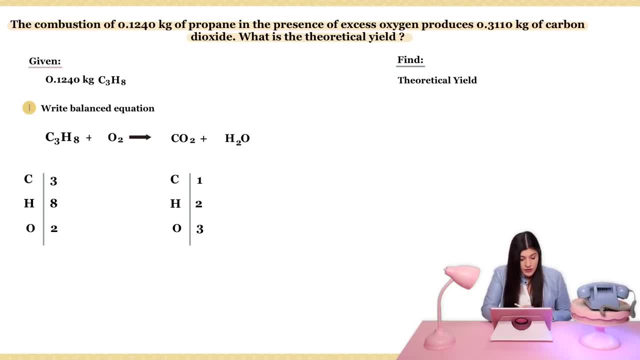 So I'm going to place a three here so I can turn this carbon into a three. So when I place a three coefficient there, what's actually happening is this is distributing, So this three is being multiplied to this one, This carbon, this three is being multiplied to that oxygen. 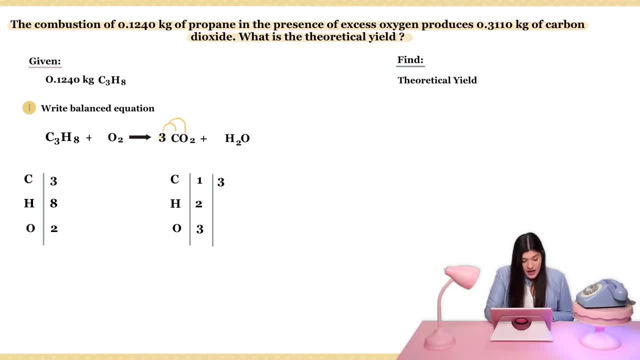 So we now have three carbons and we have three times this two subscript. We have six oxygens, but don't forget, we don't have six, We have one more. So be aware of that. So three times that, two, six plus one more. 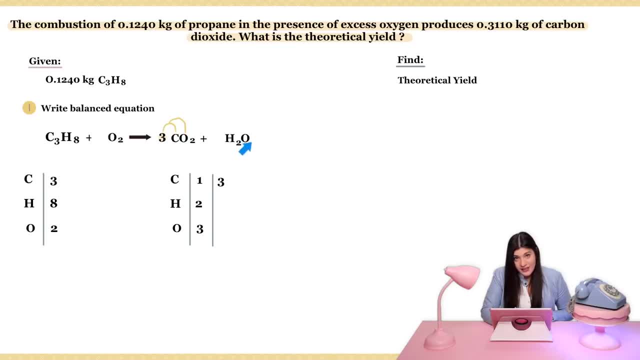 So I'd say: don't just look at one side, keep looking at like: oh, what else is this added to? Is there any other oxygens hidden there? And there are. So we have seven, So we have seven, So we have seven oxygens. 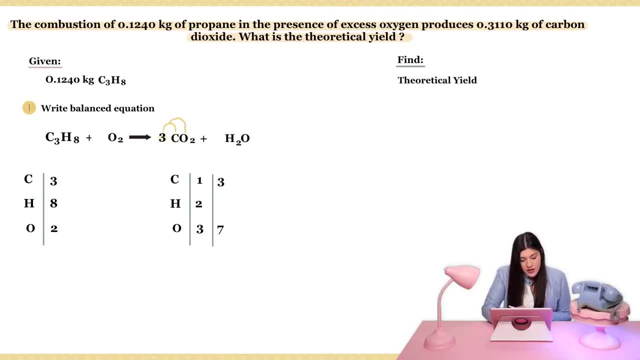 Now hydrogen. nothing changed because we didn't put anything in front of hydrogen, So that's going to remain the same as two. So now that our carbons are balanced, I'm now going to move on to hydrogen. So there's eight hydrogen here and there's two on the product side. 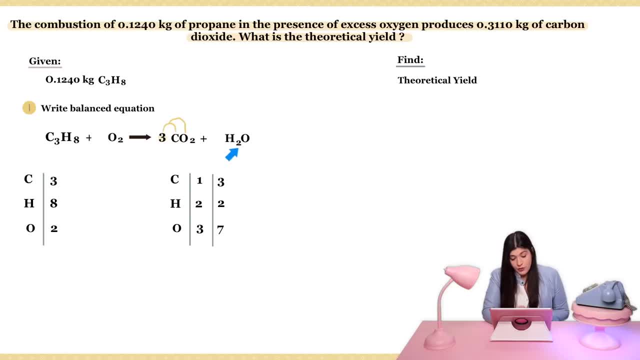 So I have to multiply a number here to two to give me eight, and that's four. So I know four will be placed there. Once again, I'm distributing this, so distribute, distribute And then. so four times two gives me eight. 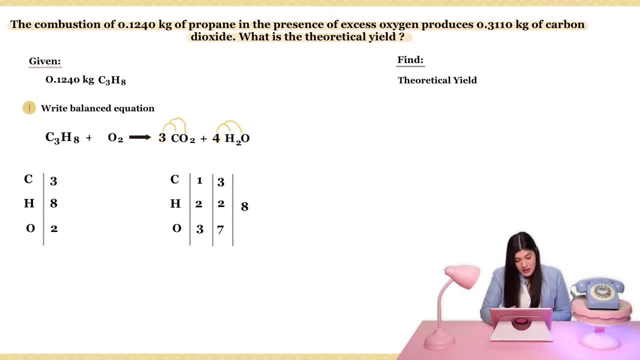 So now I changed my amount of hydrogen, So that's eight, And then the amount of oxygen will also change. So we have four here, and then plus the additional six here. So six plus four is 10.. So I have 10 oxygens and nothing changed with carbon. 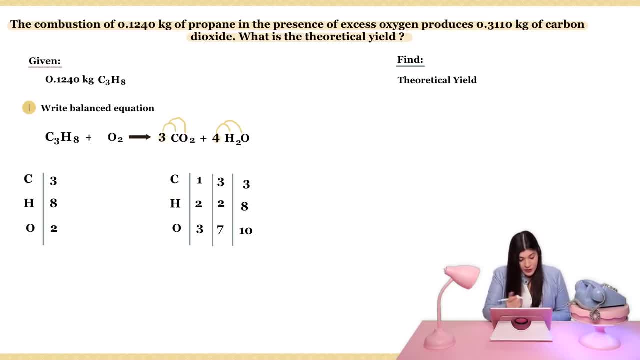 I didn't change this number, So that's going to remain the same as three. Okay, So almost there. Now we're, we're finally balanced with carbon and hydrogen. Now our oxygen is the last thing, So I have to place some sort of value here. 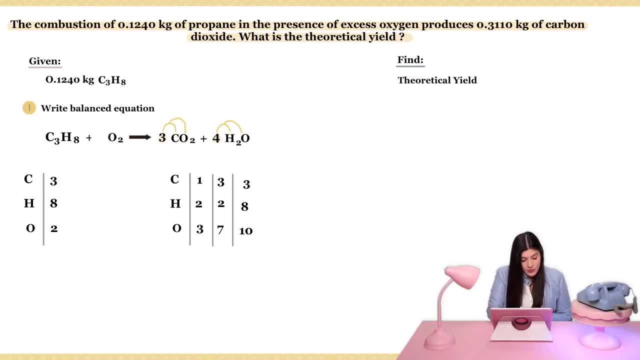 It's: multiply with two, It gives me 10.. So five times two will give me 10.. So I'll place a five And then from here this is now 10 and everything is balanced, since I didn't change anything on this carbon or anything to this hydrogen either. 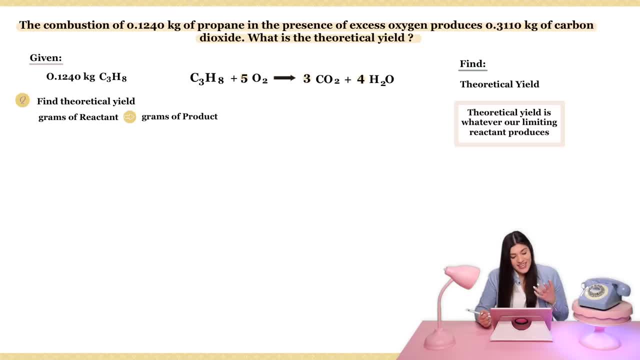 So this is our balanced equation. Continuing on. our next step is to simply find the theoretical yields. So this is really similar to the previous question with finding the theoretical yields. It's pretty much the same exact way of doing this where I'm going to convert the kilograms. 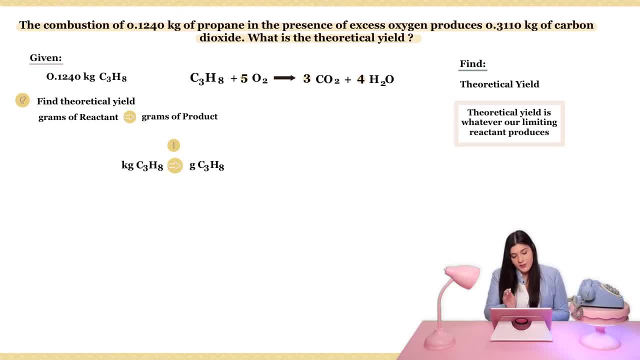 to grams. Now, after I use the metric system, of course, to go from kilograms to grams, I'm then going to use the molar mass of propane and convert this from grams to then moles. Then, continuing on with moles, I now have to change the compound. 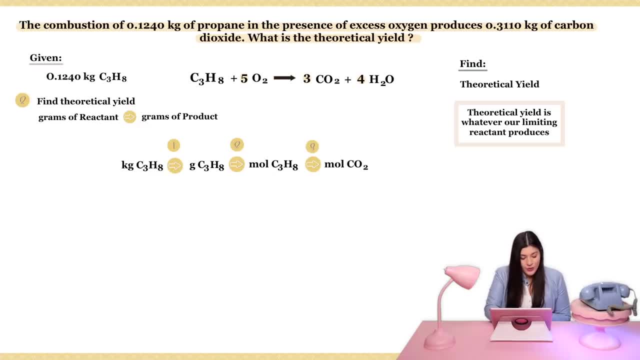 So I have to do a mole to mole ratio and that'll bring me to moles of carbon dioxide And lastly, I want to convert this to grams of carbon dioxide. So I'll use the molar mass of carbon dioxide to get to grams of carbon dioxide. 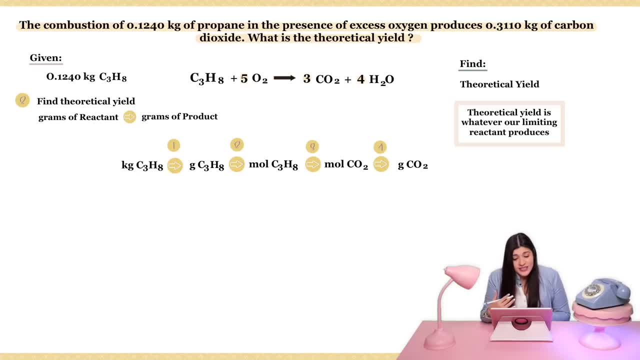 So the theoretical yield, I know, is whatever The limiting reactant produces. our limiting reactant in this case, because it really tells us, is propane, since our excess reactant- hint, hint, excess- is oxygen. okay, is that O2.. So, okay, I know that, since that's given, I don't have to do this twice. 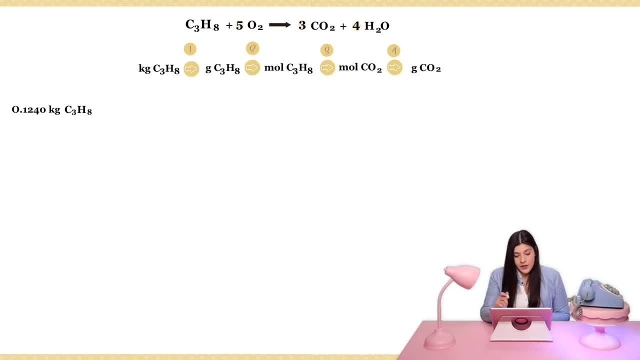 And let's keep going with this. So I'm just going to put this all together, So, starting off with what we're initially given, the kilograms of propane, and I want to convert this to grams. So, once again, I'm going to convert this to grams. 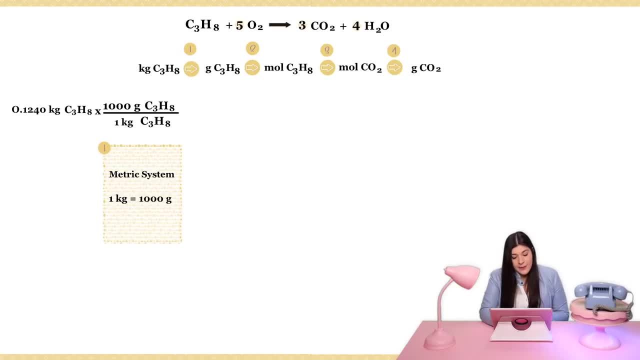 And I'm just using the metric system, which was that one kilogram is equal to 1,000 grams, Aligning our units across from each other, so they can cancel. So this cancels, this cancels. We're now at grams of propane. 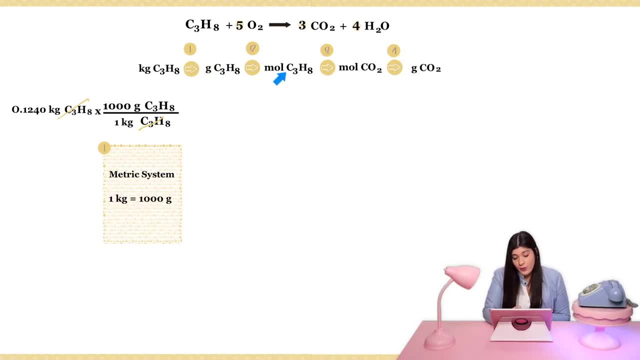 So I'm here. Next, I want to move on to moles of propane. How do I go from grams to moles? I use the molar mass. So I need to find the molar mass of propane, which is what I did here, multiplying that. 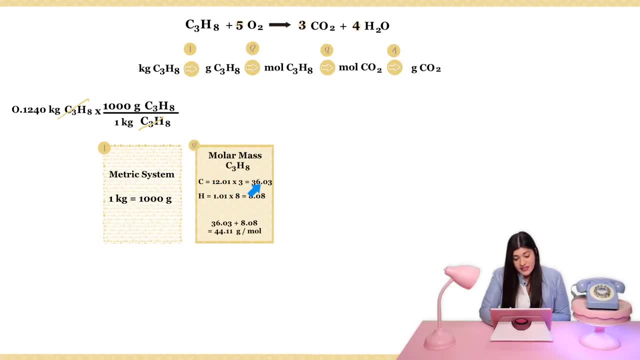 12.01 times the three subscript to give us this. Next, multiplying 1.01 times that eight subscript to give us this: Add these two values together and 44.11 is our molar mass of propane. So of course, once again, I want to align the units so they can cancel. 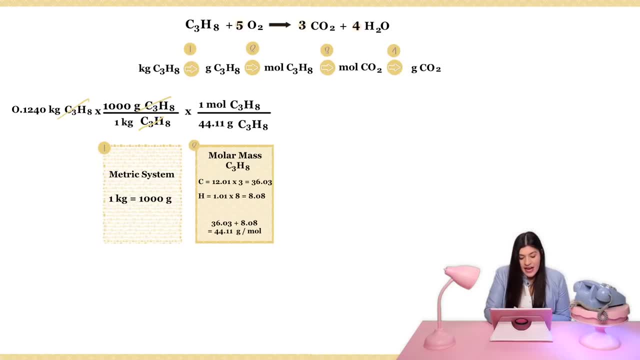 So these two grams across from each other so they can cancel out. And I'm now at moles of propane. So I'm here at this step. Now I want to change the compound. So when I want to change the compound, I'm going to use a mole to mole ratio which is 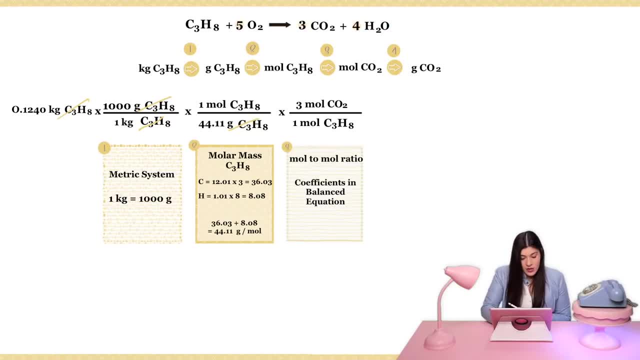 found using our balanced equation. Okay, I want to align my units so they can cancel. And remember, if we don't have a coefficient in front, then assume that it's just one. So in this case, I know that for one mole of propane, which I'll align the units. so 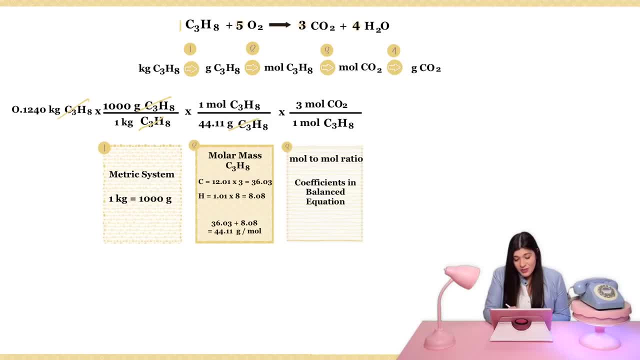 they can cancel. there's three moles of carbon dioxide, which is on top, So our units of moles of propane will cancel. And then next I'm here, So I just have to convert this to grams of carbon dioxide by using the molar mass. 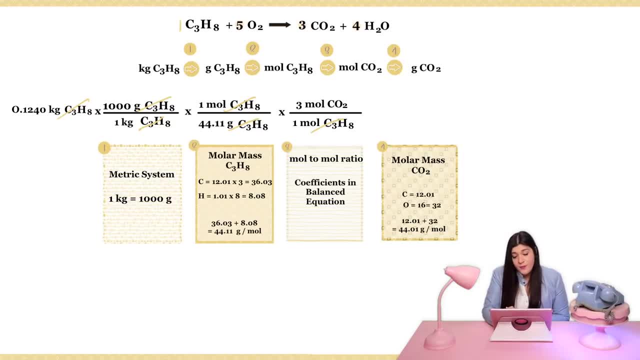 So, remember, molar mass allows us to go from grams to moles or vice versa, moles to grams, And then identifying the molar mass of carbon dioxide. we did that previously, And all I have to do is then align the units again so they can cancel. 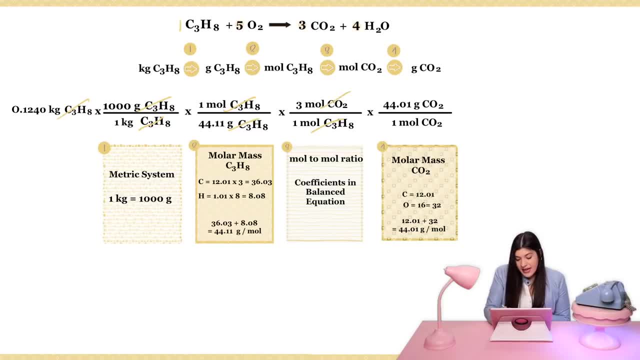 Moles of carbon dioxide are on the bottom. Those would then cancel out to get grams of carbon dioxide And we're just going to multiply everything on top, So all of these out, and then divide it by that 44.11. And it's going to give us this value. 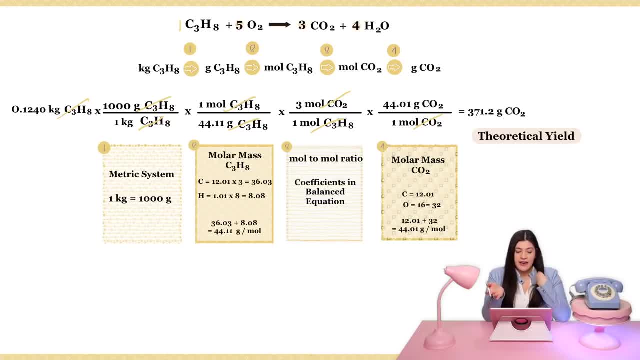 We could stop here. That would still be correct, But because they gave us the amount of kilograms- Okay, The amount of kilograms in general, right, Everything was initially in kilograms. They most likely want the answer to remain in kilograms, So I'm going to convert this back down to kilograms. 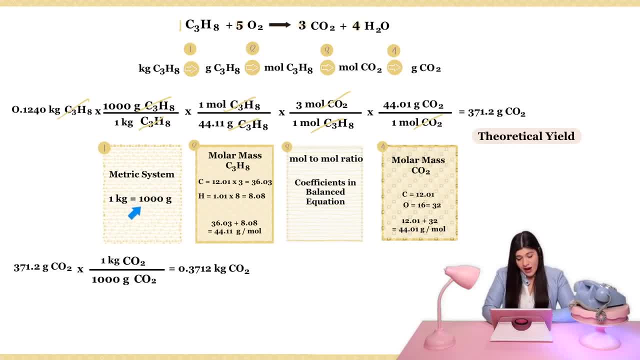 And all I have to do is using that metric system again, right? this conversion factor is: align those units across so they can cancel. So I'm dividing by 1,000.. And then that's going to give me this amount of kilograms overall. 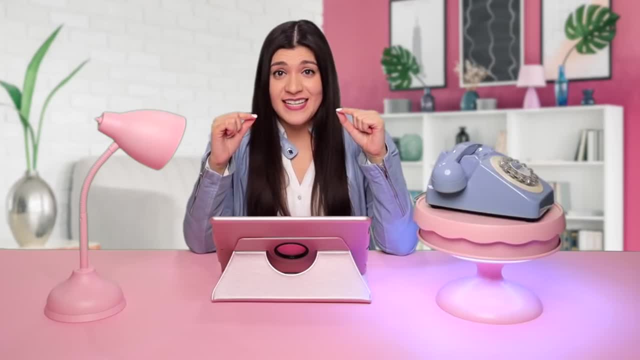 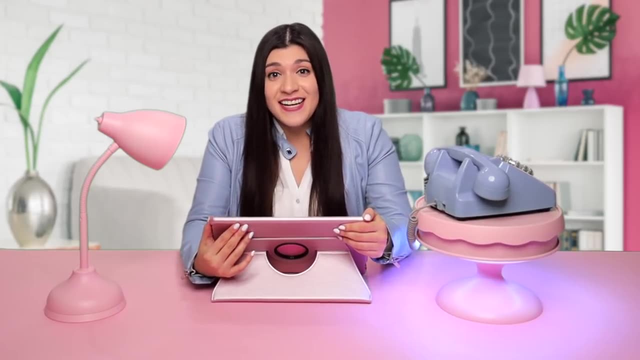 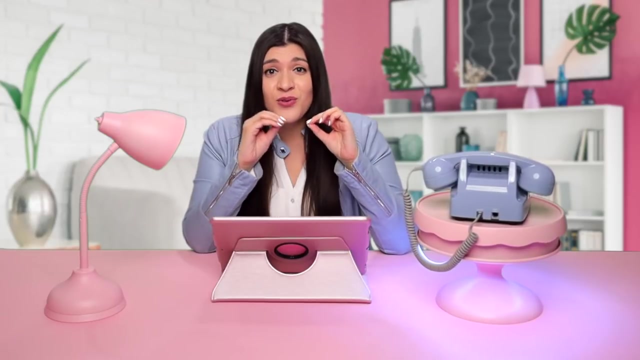 So this is my theoretical yield. This question is a common test question and a finals exam question. Yeah, I know, So make sure to study these types of questions. Anything talking about percent yield, theoretical yield, limiting reactants, All of that is the most common final exam question. 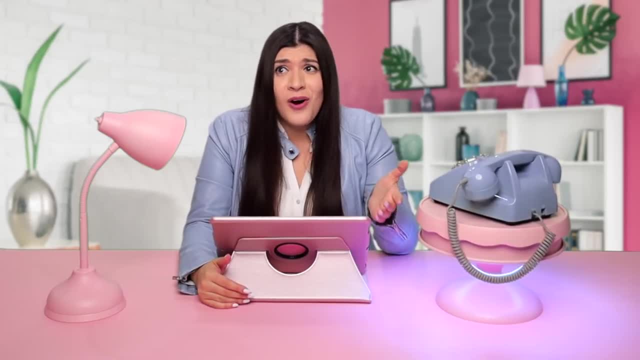 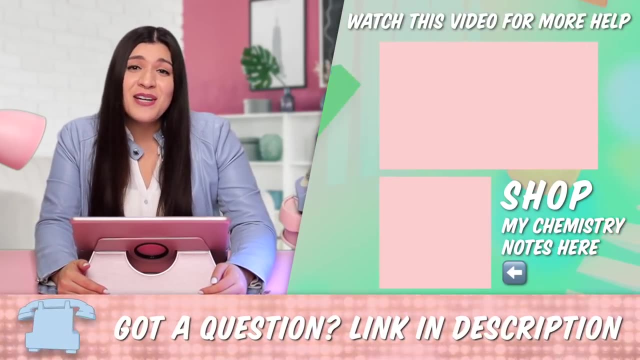 Now, if you have other questions and you want the answers to them and want to figure out what am I doing, please ask me. Simple as that. So in the description box you'll find a link And you could submit your question. And I'll be happy to answer it And I'll see you in the next video. 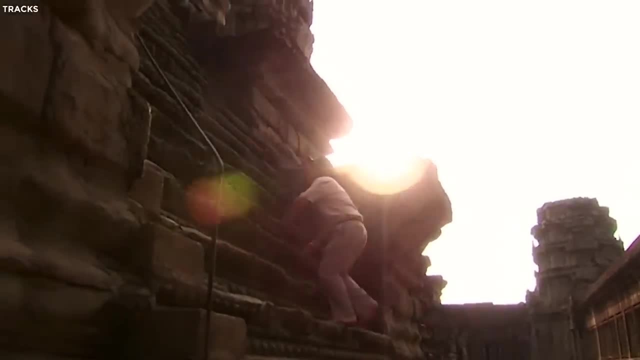 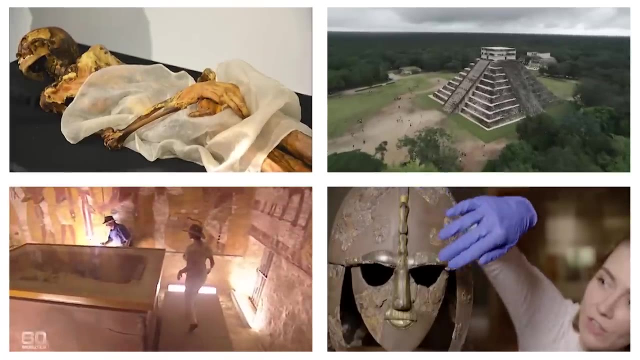 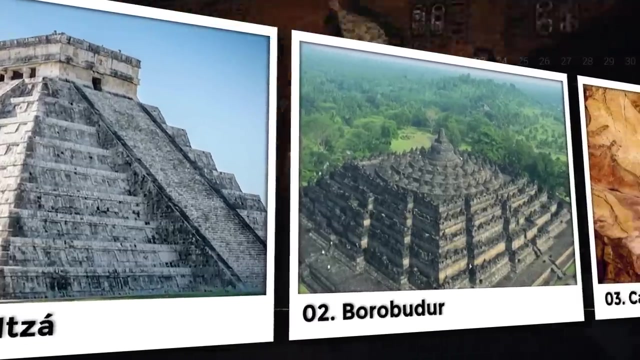 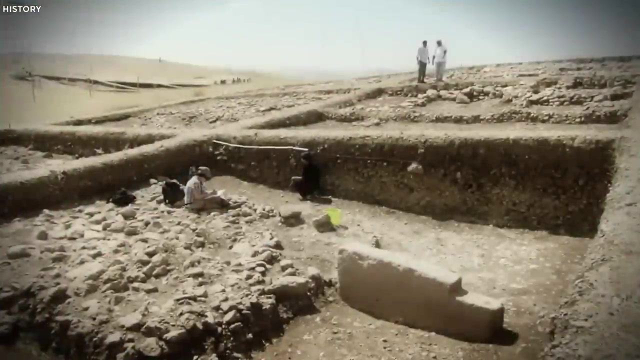 Can you believe that some of the world's most astonishing archaeological discoveries were made completely by accident? Join us as we take you on a journey through history and explore the top 20 greatest archaeological discoveries of all time, From the discovery of the Dead Sea Scrolls to the stunning unearthing of Machu Picchu. 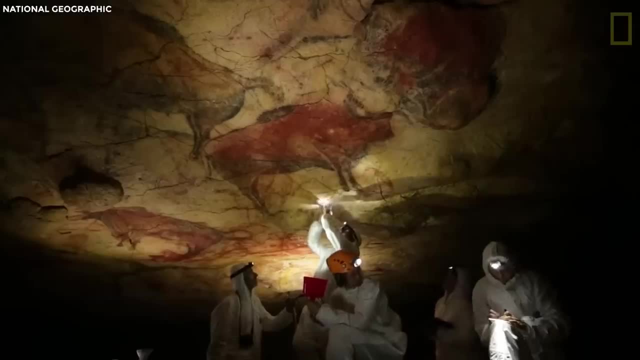 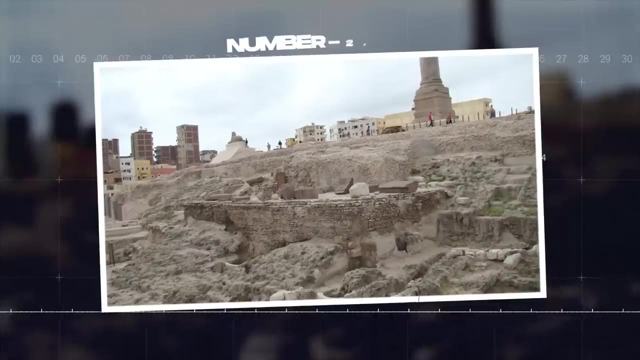 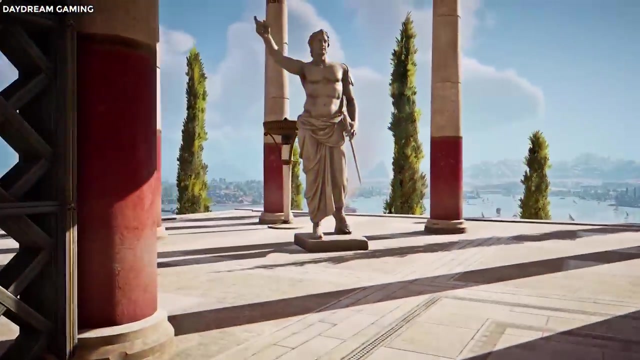 we will uncover the fascinating stories behind these incredible discoveries and the secrets they reveal about ancient civilizations. 20. The Serapium of Alexandria. First off, we have the Serapium of Alexandria. It's not a name that exactly rolls off the tongue. 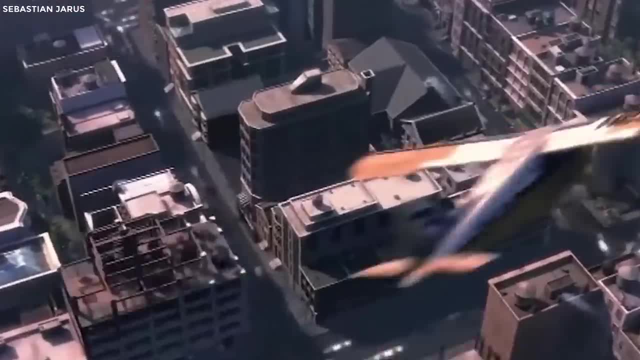 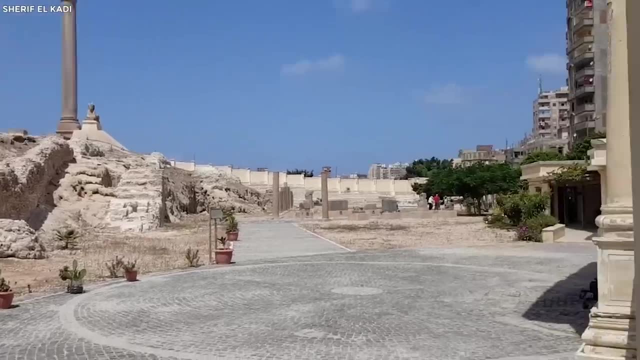 but it's a place that will leave you tongue-tied. Let's travel back in time to the year 1850, when Auguste Mariette, a French archaeologist, stumbled upon the Serapium of Alexandria completely by chance It had been buried. 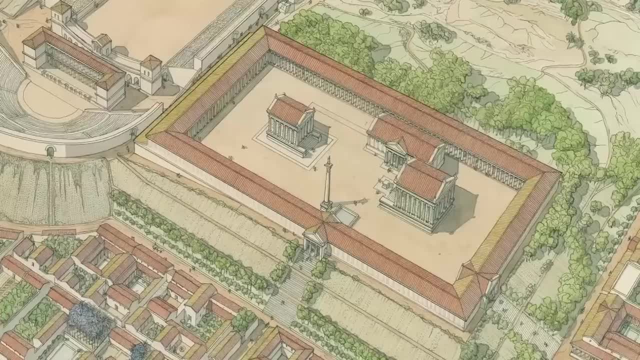 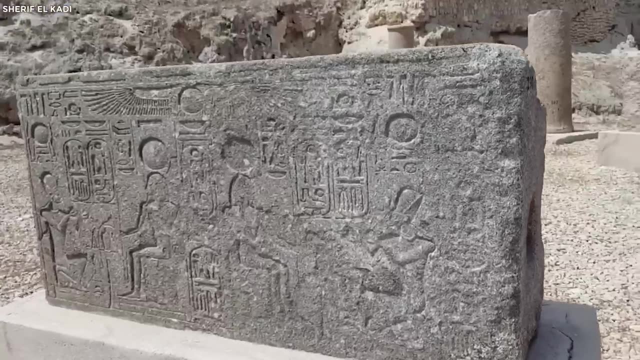 and forgotten for centuries before Mariette's discovery. The grandiose complex spanning over 30,000 square meters, with towering columns and intricate carvings, would have been enough to make any archaeologist's heart skip a beat. But what truly caught Mariette off guard was 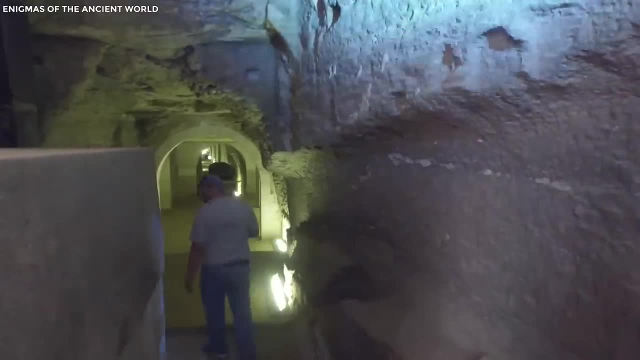 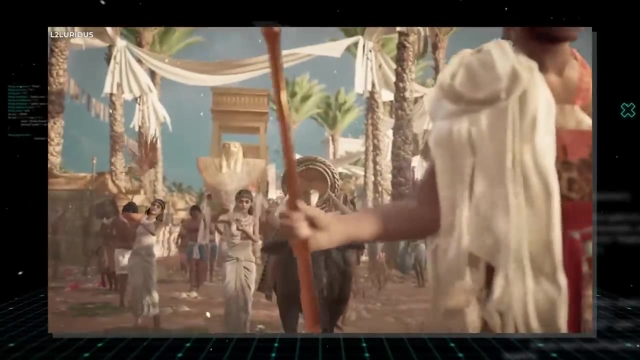 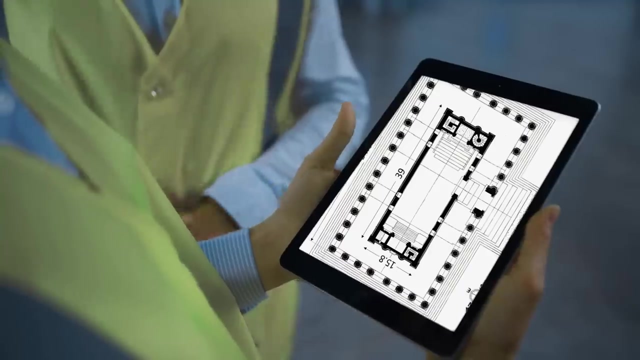 the fact that this temple was essentially an underground burial chamber for bulls. Yes, bulls. The worshippers of Serapis believed that these animals held the key to the afterlife, or perhaps were just very fond of their beef. Despite the absurdity of it, all the engineering. 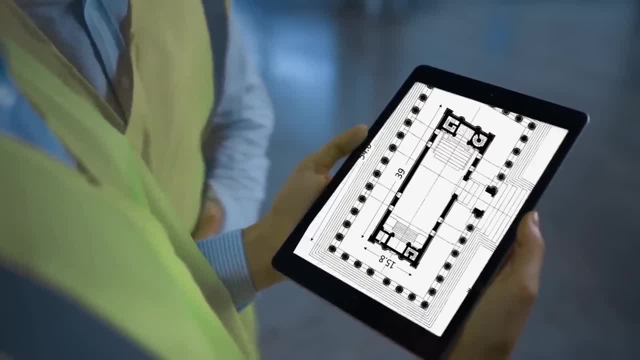 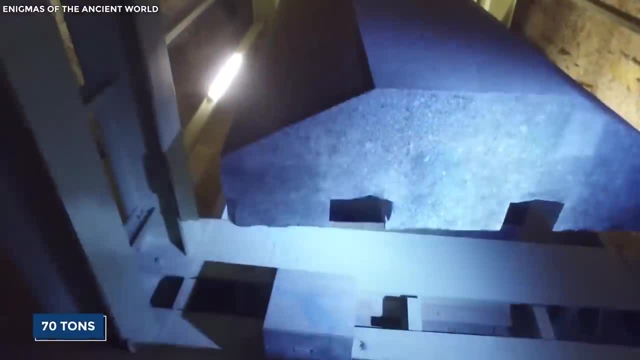 feats achieved in the construction of the Serapium cannot be denied. The network of underground tunnels lined with massive granite sarcophagi, each weighing over 70 tons, is a testament to the ingenuity of ancient engineers And the mystery of the Serapium of Alexandria.